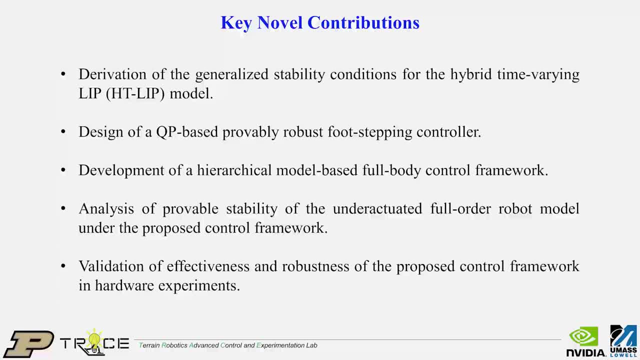 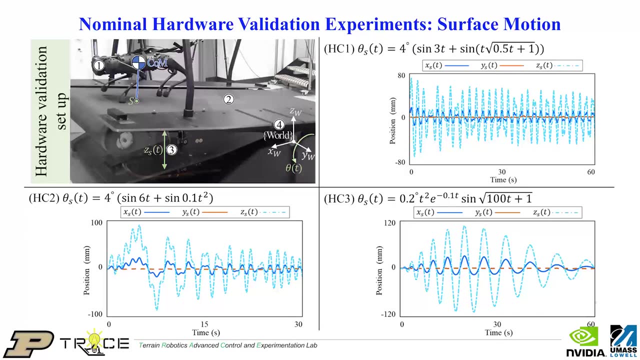 footstepping controller. developing a hierarchical model based full body control framework. analyzing the provable stability of the full order robot model within this framework and validating the effectiveness and robustness of the proposed control framework. Here we show the hardware validation setup: nominal general motion profile of a point near the robot on the treadmill. 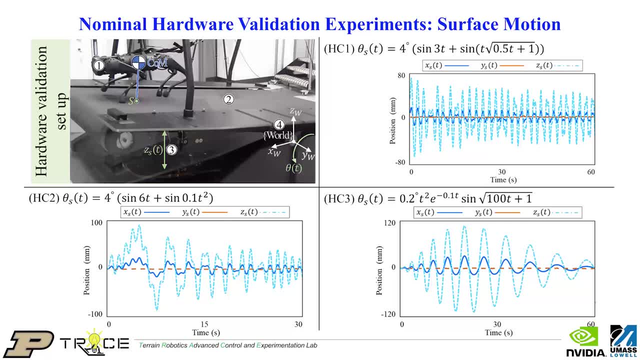 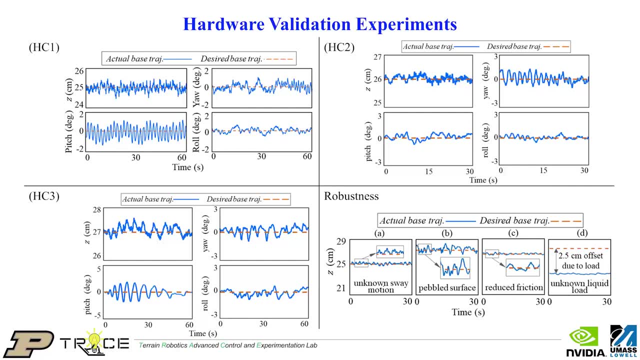 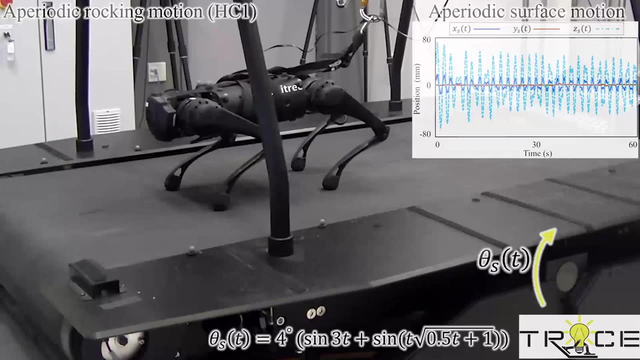 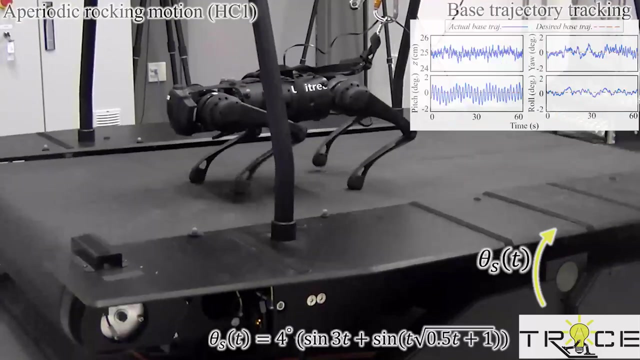 and corresponding results of desired trajectory tracking. During hardware experiments. the corresponding base pose tracking illustrates reliable trajectory tracking supporting stable quadrupedal trotting on surface with general vertical motion. The hardware experiments for these cases confirm stability. In all cases the motor torque shows a consistent profile respecting the torque limits. 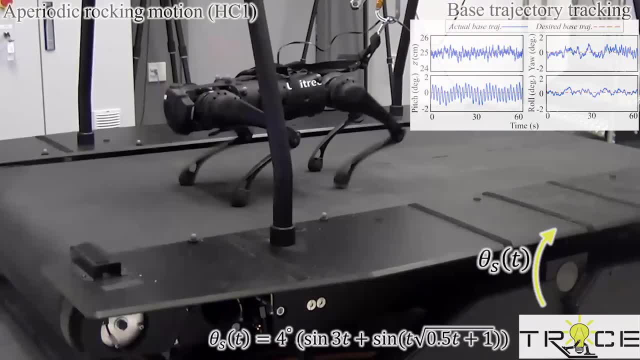 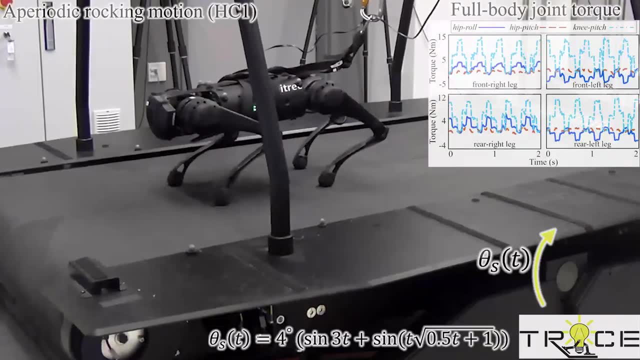 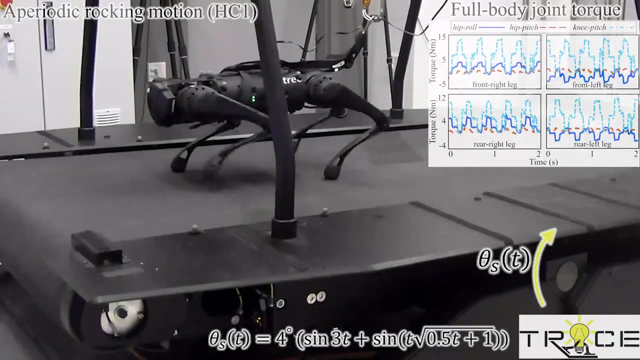 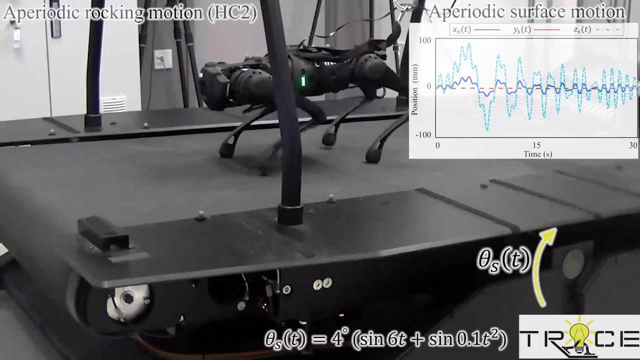 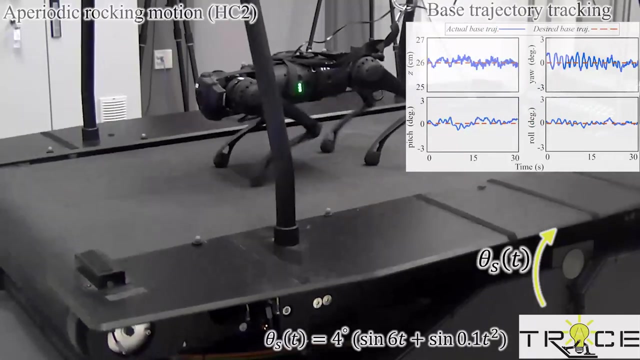 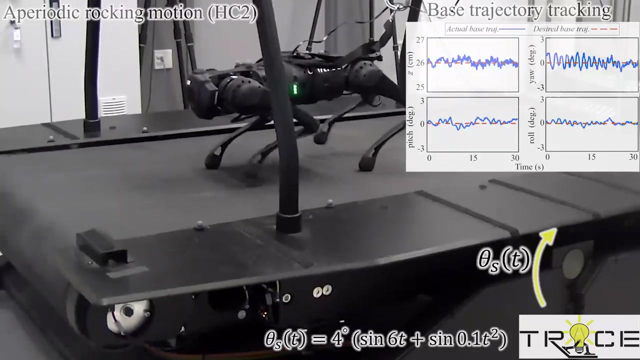 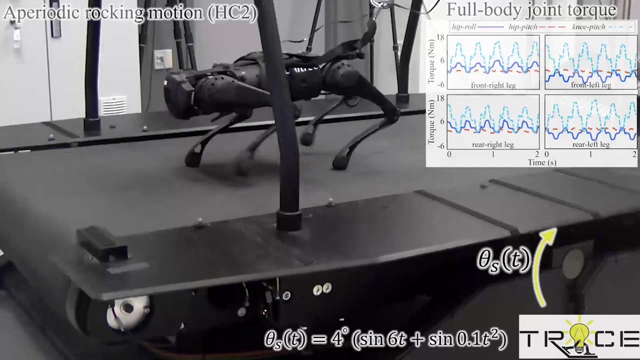 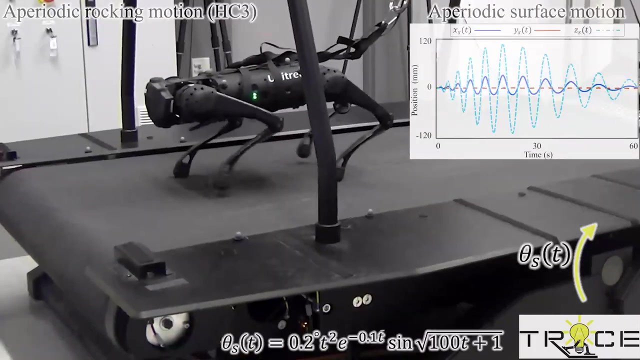 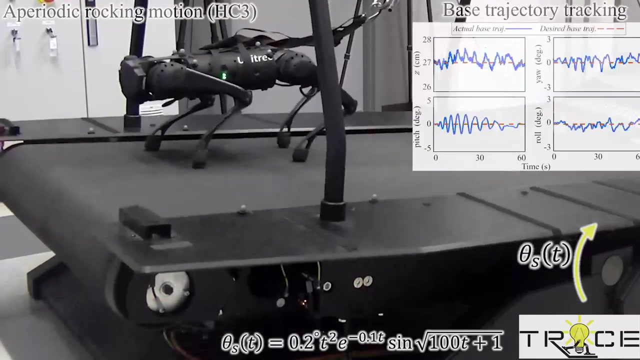 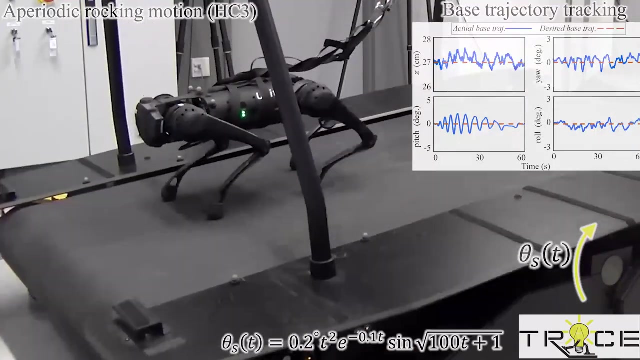 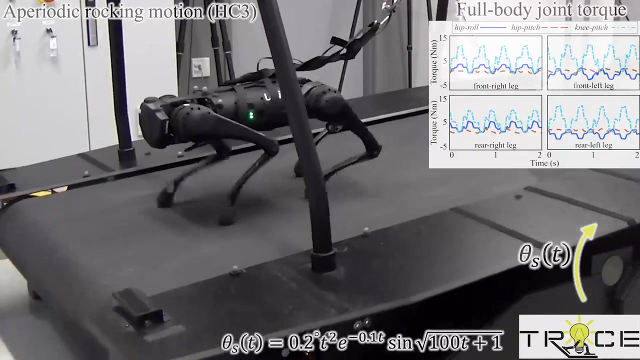 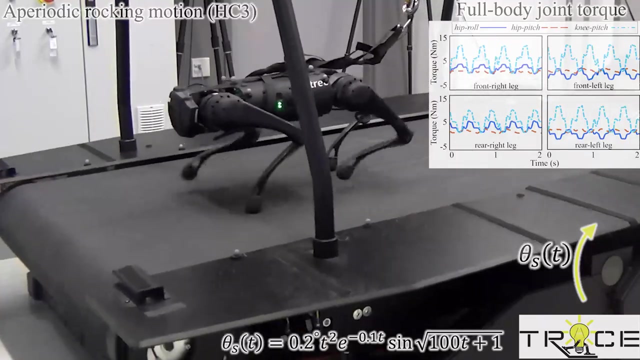 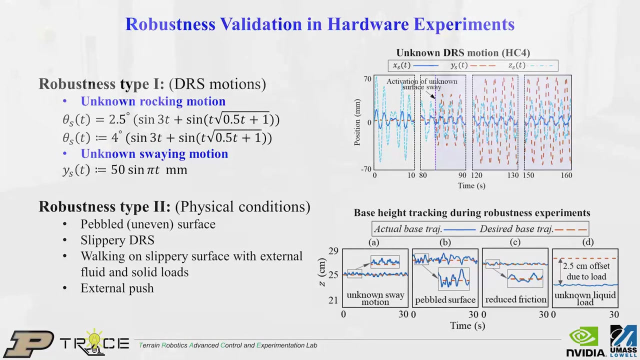 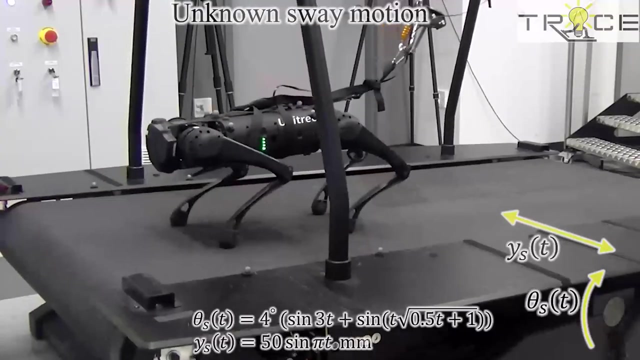 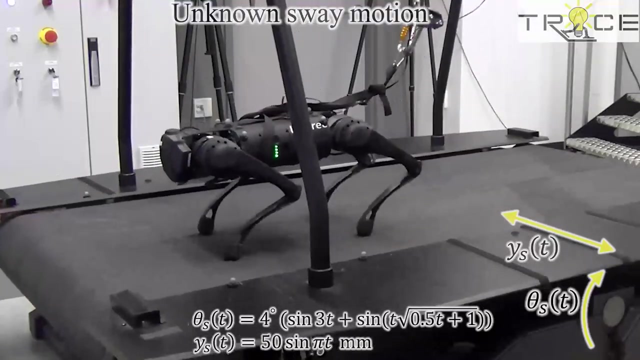 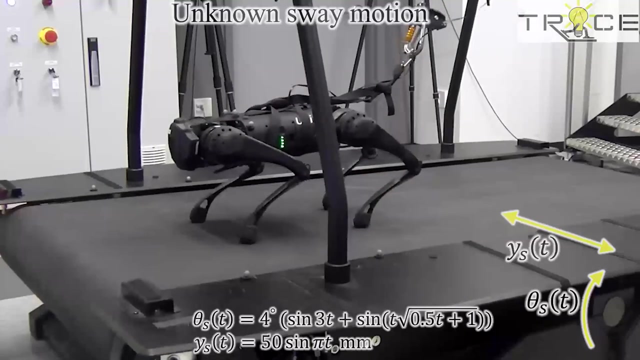 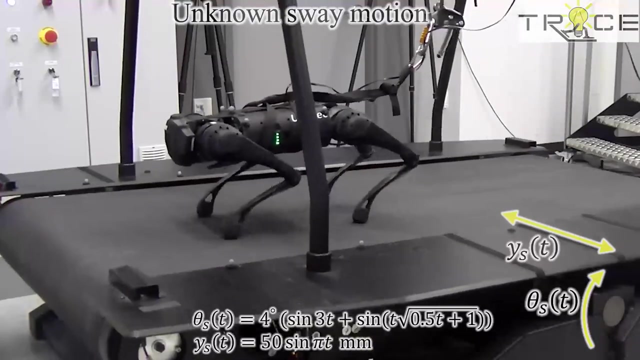 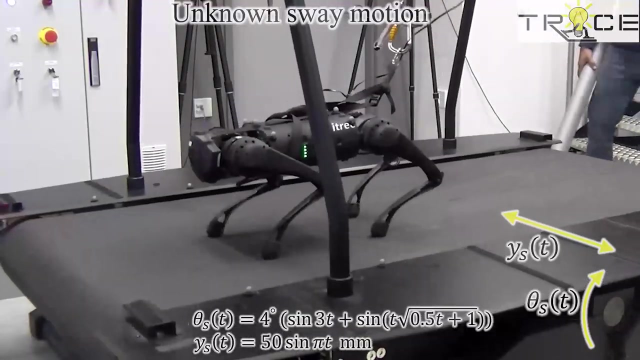 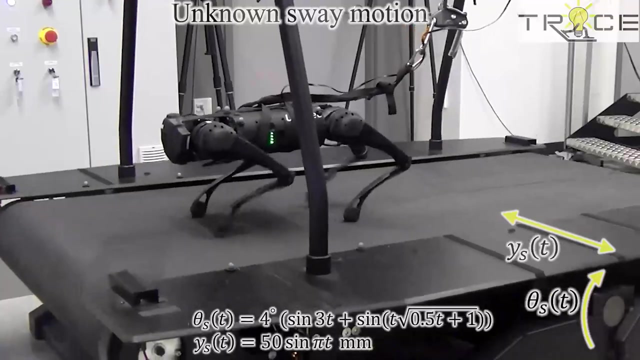 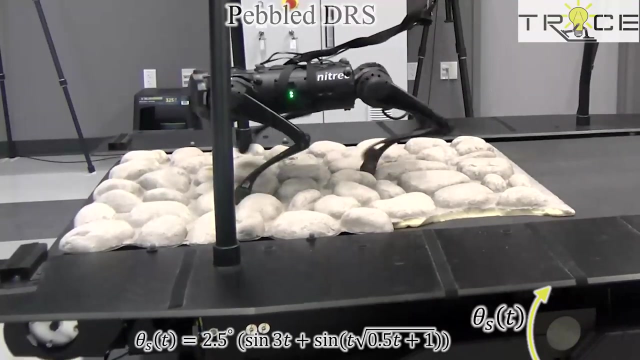 The Thank you. In addition to the nominal cases, we also validated robustness under various uncertain cases. In all cases of robustness expectations, the uncertainties are effectively handled and the robot sustained stable trotting, as evident from the base height tracking results. In all cases of robustness expectations.